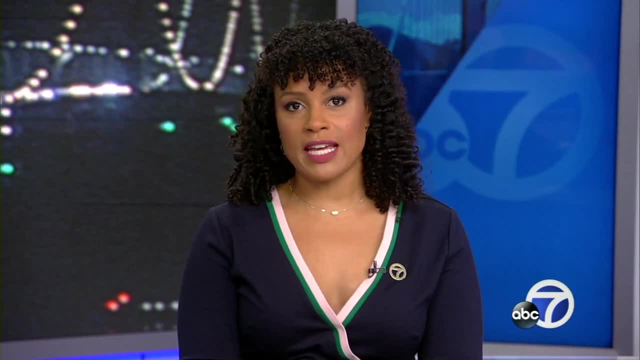 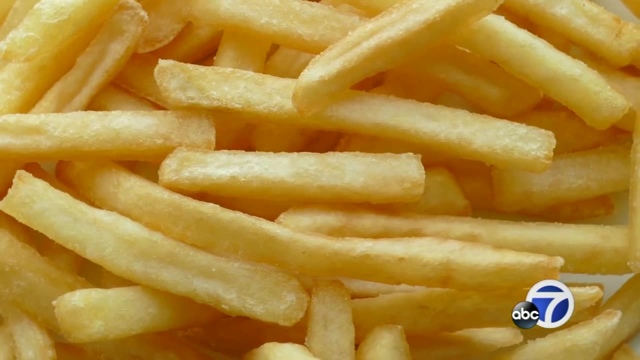 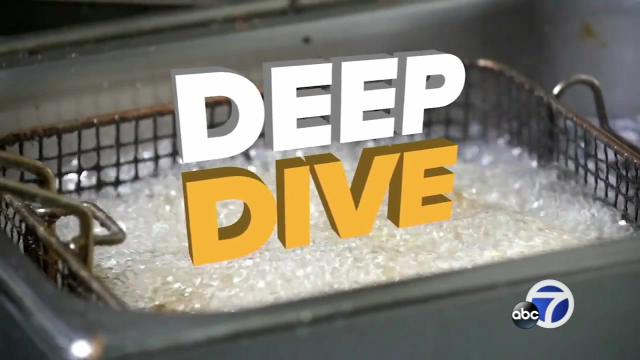 The upcoming new year means plenty of new laws coming into effect in California, but one may affect your day-to-day the most. The change could have a sweeping effect on the fast food industry in the state. So we're making it tonight's ABC 7 Deep Dive at 11 to dig deeper on an issue impacting you. Tonight, ABC 7 News reporter JR Stone takes a closer look at how a new minimum wage law could shake up your next order. 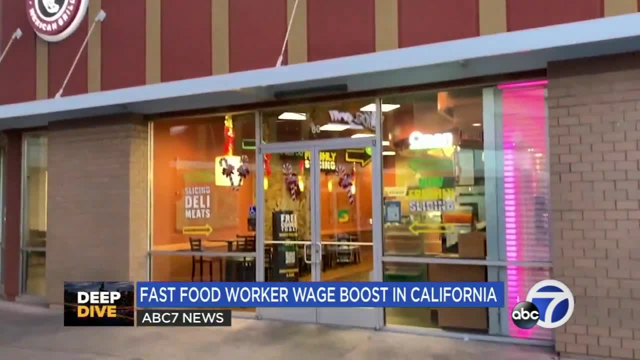 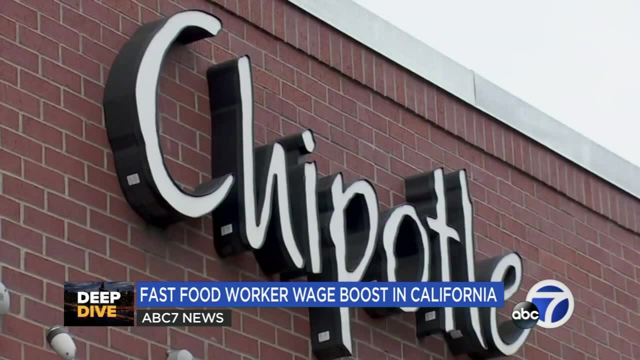 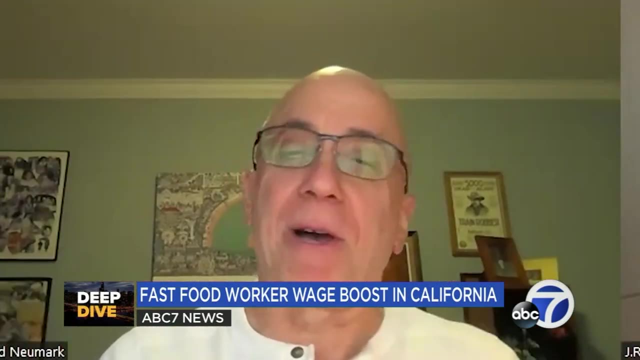 California workers at most fast food chains with more than 60 locations will make $20 an hour starting on April 1st 2024.. It's a new law. An economist that we talked with said it will affect you Higher prices, but that's not all. 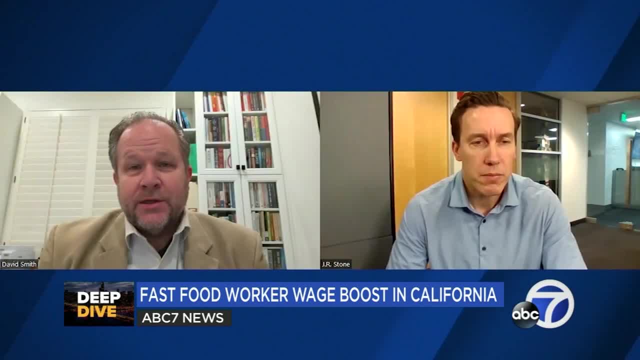 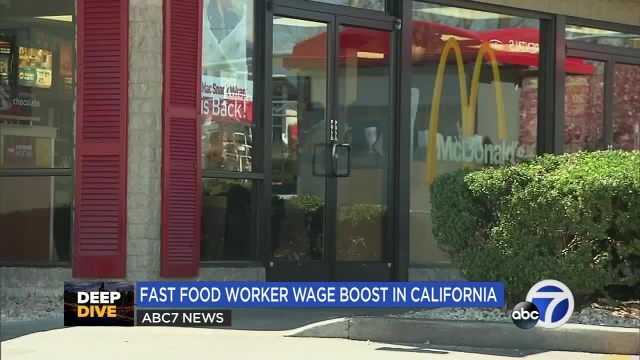 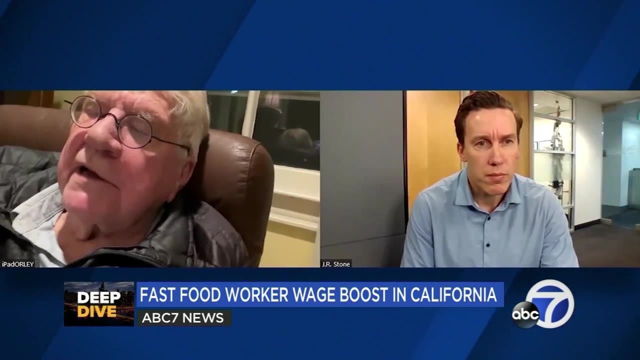 We asked three economists, professors from elite universities across the country, including Professor Orly Ashenfelter at Princeton University, who studied minimum wage increases at McDonald's and published his study in 2021.. If the wage goes up by 10%, the price goes up by 2%. 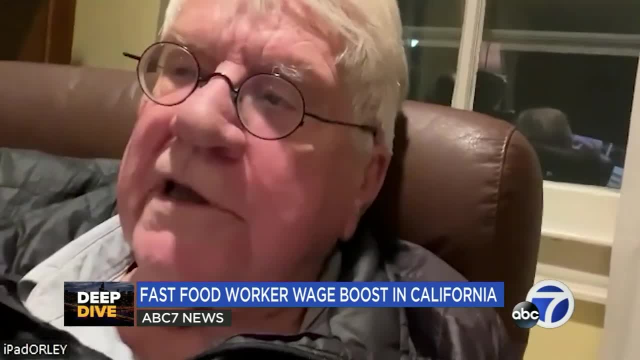 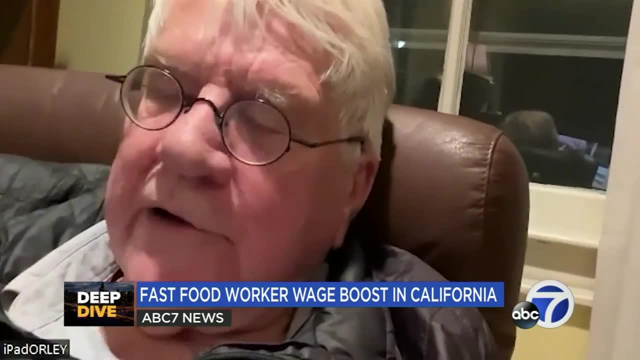 We're on a projection. This is based on the fact. It's on the history. Historically, when minimum wages go up, about 20% of the increase is passed through in prices. That's the way it's been for decades. 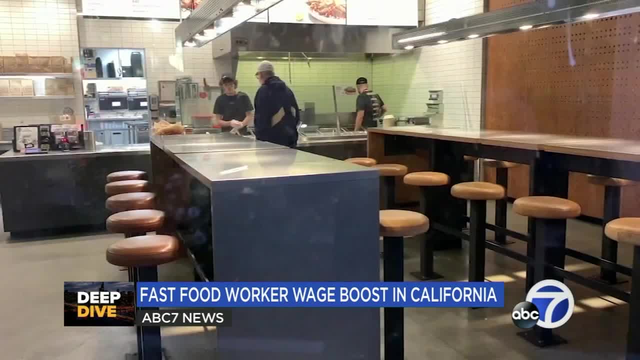 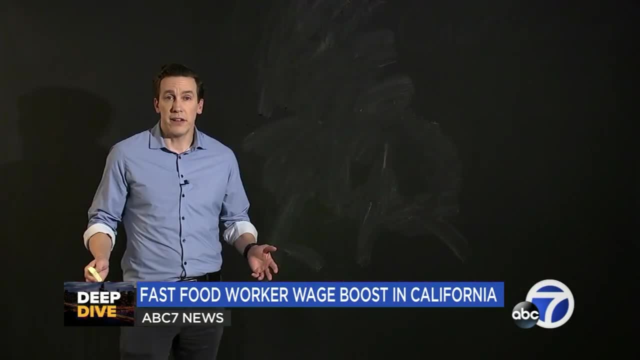 McDonald's and Chipotle both announced earlier this year that prices will go up in California when this takes effect, But they haven't said by how much. Each food restaurant is different, But let's just say they're paying somebody $15.50 an hour. 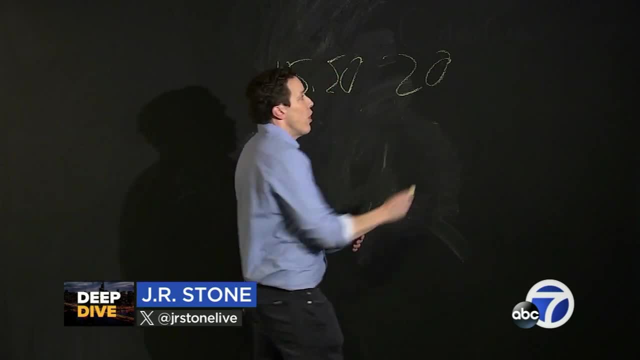 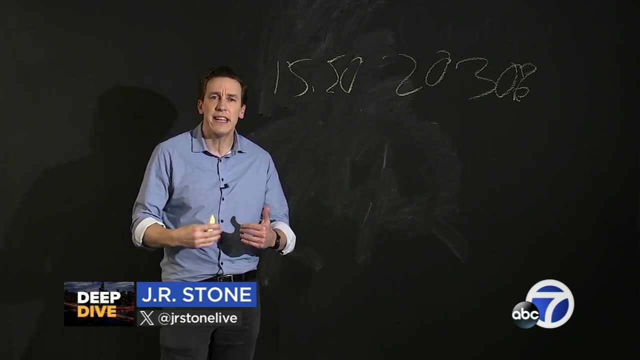 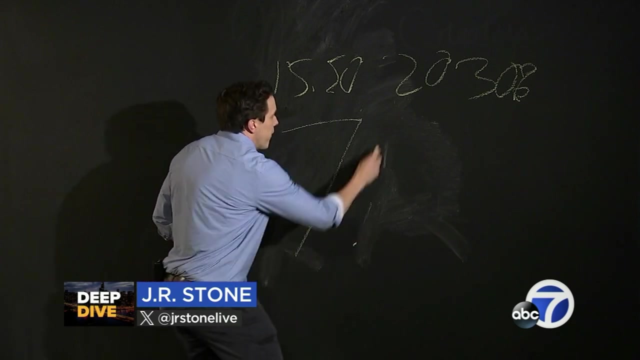 Now they're paying somebody $20.. Which is a 30% or nearly a 30% increase. Orly, who you just heard from there, says you'll likely pay an additional 6%, So that Big Mac that was going for $7 is now going for $7.42.. Or likely to go for $7.42.. But that's just one of the changes we could see. Some estimates suggest that we could have up to 50,000 jobs lost in the state of California. I do. You could have longer lines. 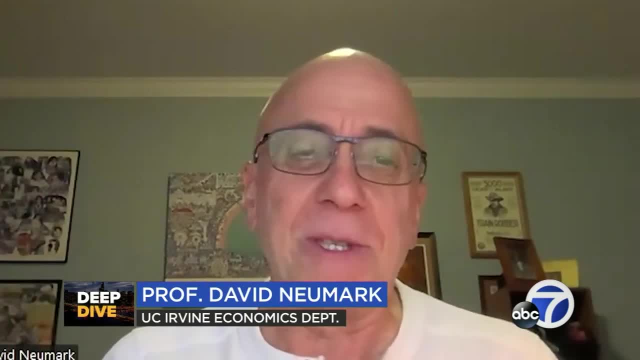 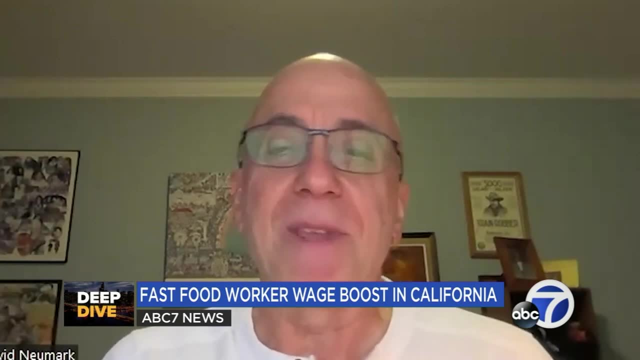 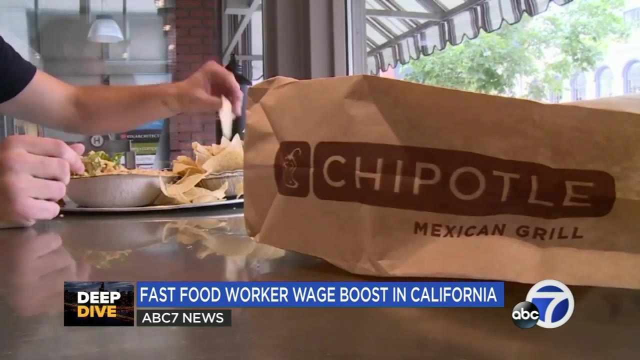 You might have dirtier restaurants. There's even a study from Seattle. when they raised the minimum wage, Hygiene violations increased. But consumer prices is also one potential route. What makes the increase easier for businesses is that all the chains will likely raise their prices. 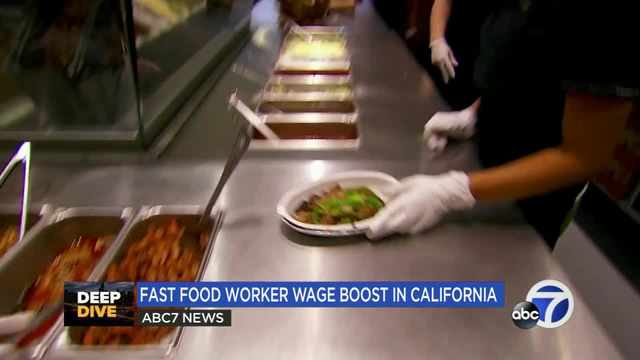 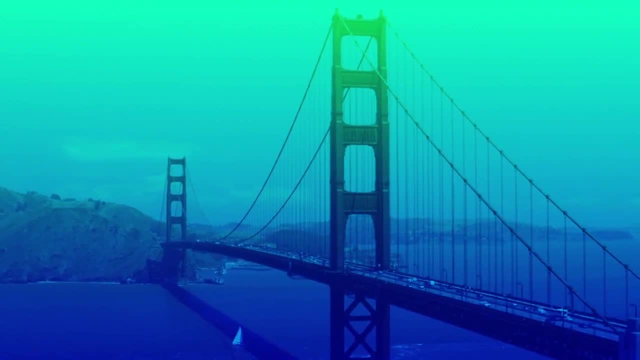 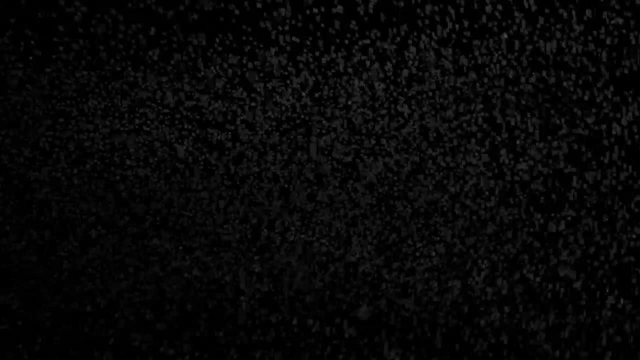 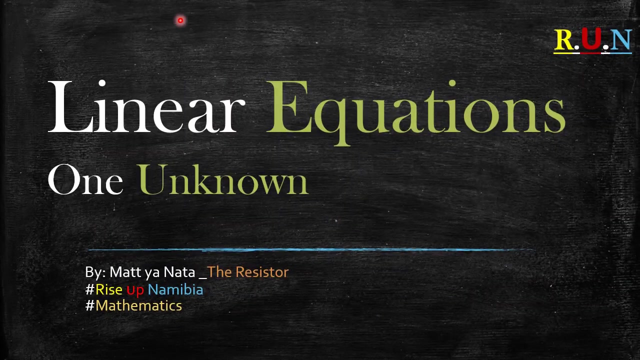 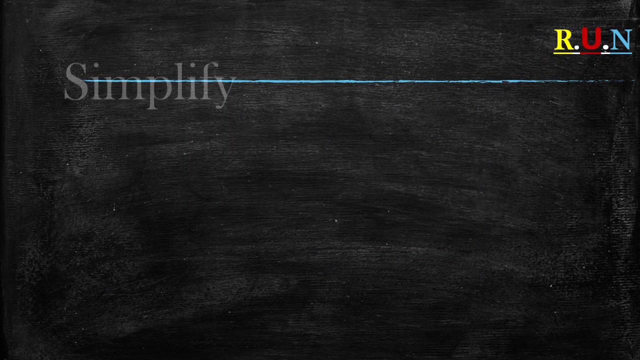 Welcome to Rise Up Namibia. So in this video we're going to be looking at linear equations involving one unknown by Med Yannata, aka the resistor of bad and the lover of good. hashtag: dark and lovely. underscore: walk by faith and not by sight. So to explain this,